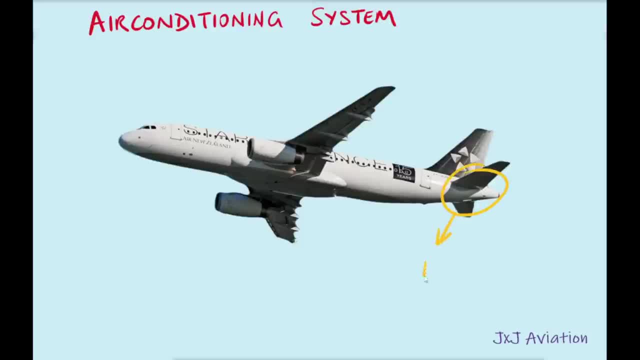 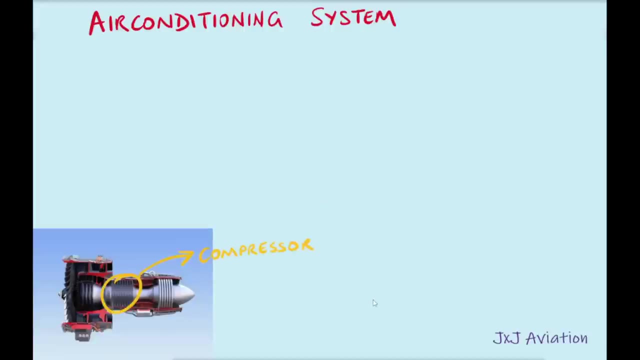 The air for the air conditioning system is taken from the auxiliary power unit or the engines. When the engines are running, bleed air is taken from the compressor section of the engine. The air flow is controlled by a control valve. This air will be too hot for the system to handle. 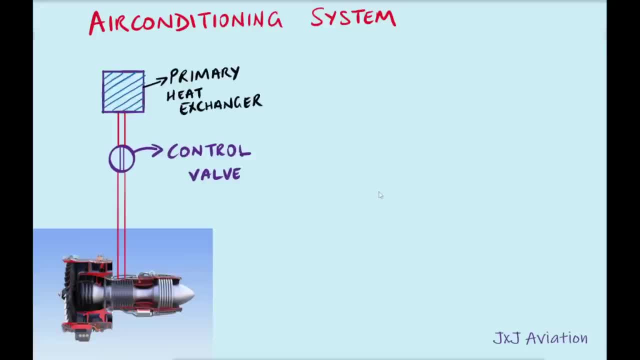 So it is sent through a primary heat exchanger. This is an air to air heat exchanger where cold air is taken from the engine's inlet section. This air is then sent to an air cycle machine. This air cycle machine is mainly responsible in providing cold conditioned air to the aircraft. 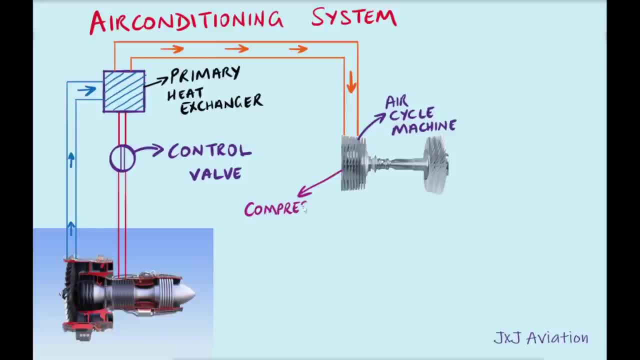 The air cycle machine consists of a compressor and a turbine connected to a single shaft. The air initially enters the compressor section. The compressor increases the pressure of the incoming air, But along with the pressure the temperature of the air will also increase. So the air is passed through another heat exchanger, called the main heat exchanger. 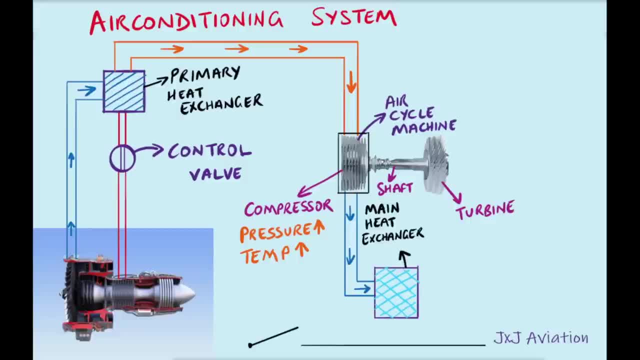 This is also an air to air heat exchanger which uses the cold outside air called as ram air. This air is taken into the aircraft by a ram air inlet, passes over the main heat exchanger and gets discharged overboard. The air then enters the turbine section of the air cycle machine. 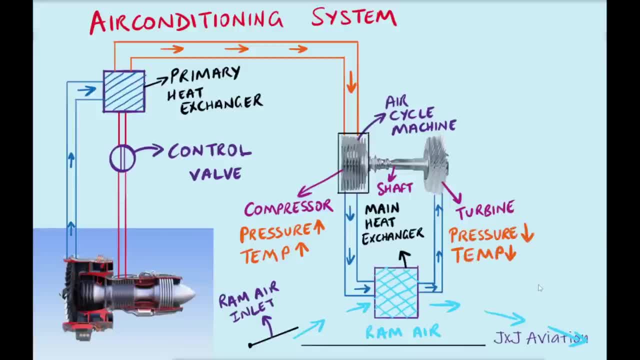 Here the air gets expanded, which means the pressure of the air reduces and with it the temperature reduces further. This is the cold conditioned air which is sent into the aircraft cabin and the cockpit Before entering the aircraft. the water molecules in the cold air are removed by a water separator and then sent to a mixer unit.